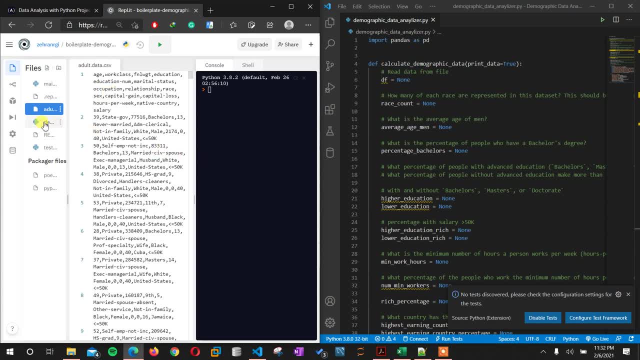 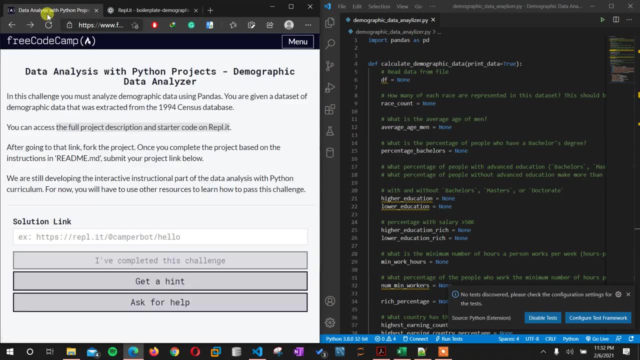 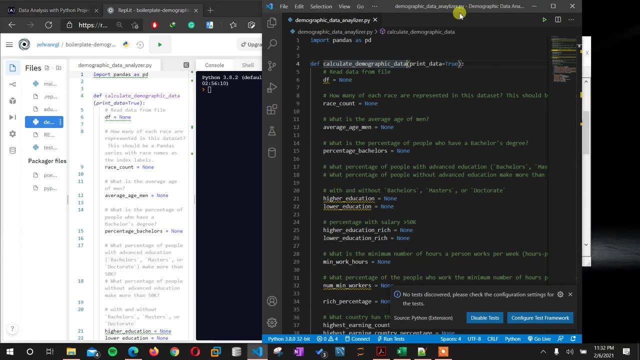 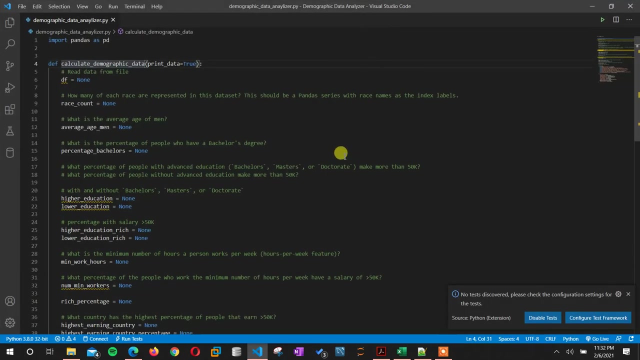 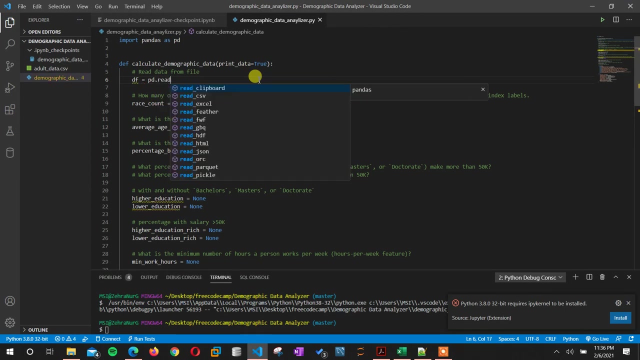 file. I'll show it and we're gonna use our test module here. Okay, so just firstly from here what they want. just come here and start from here. So firstly, we should read our file, right, So read CSV, yes, and here, that's it. Okay, it will read it, Okay. so they ask: how many of each? 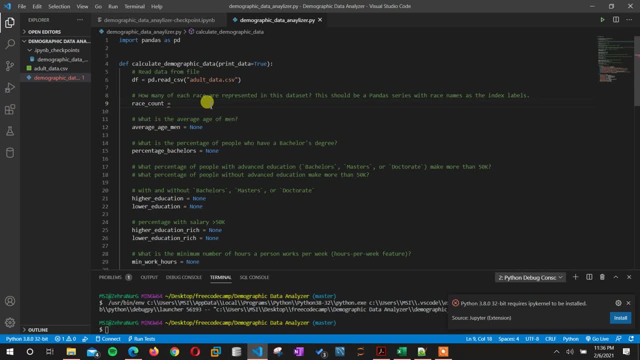 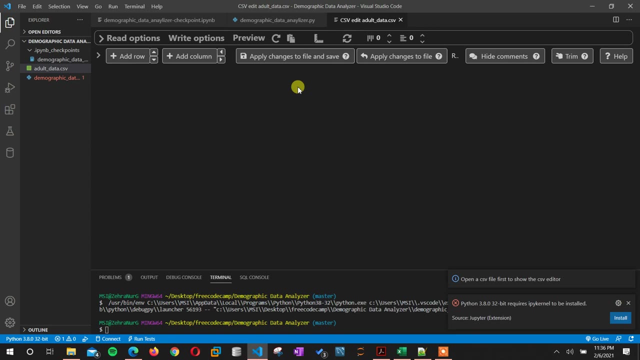 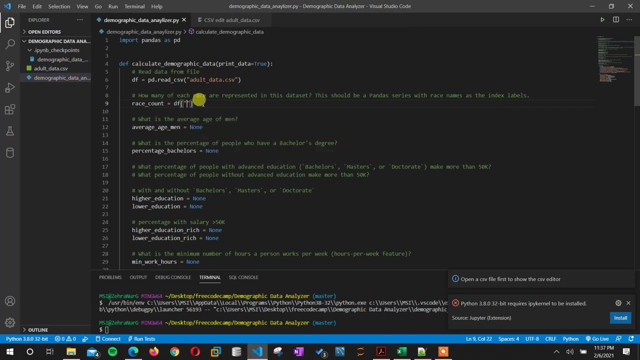 arrays are represented in this data set. So I'm just going to check the column name. Okay, so I can say I'm gonna change it. Okay, so there's my arrays here, so you can see my column name. just as they ask, I'm gonna say IDF, bring my arrays. 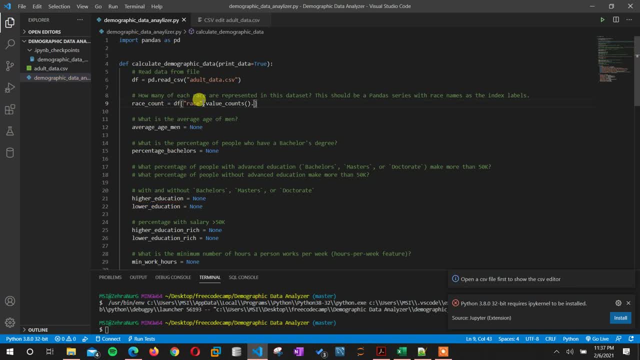 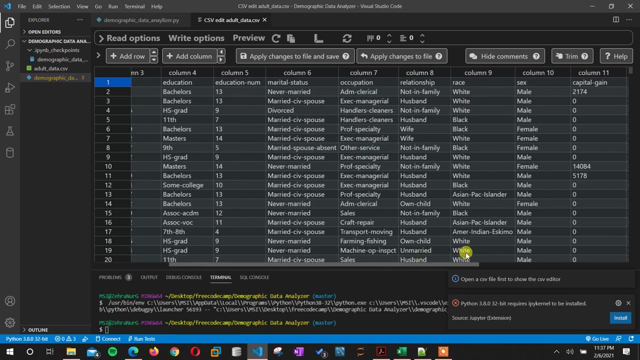 And the value, and I'm going to do it like to list, okay for it. and this is here. okay, that's it. okay. so you know, okay, that's it. what is the average of the main? okay, you can, you can actually say hi, df, df- and this is my column name here- for finding the man or female here. okay, so the important. 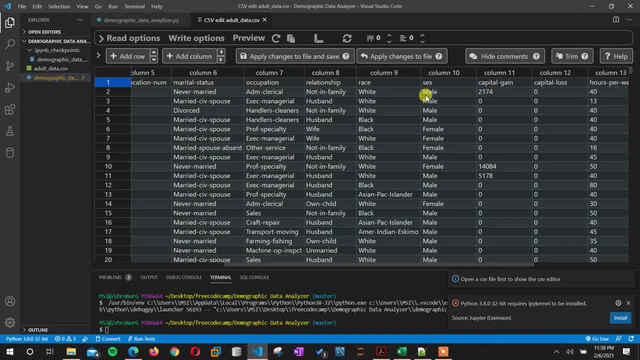 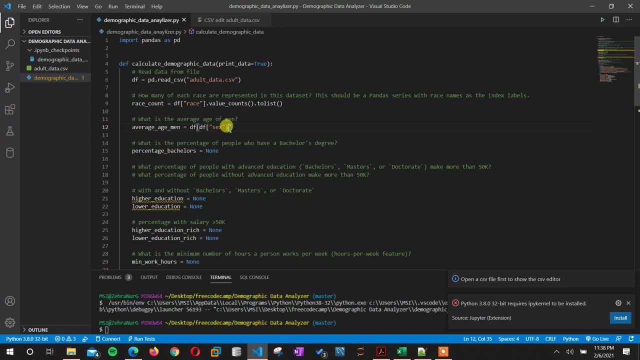 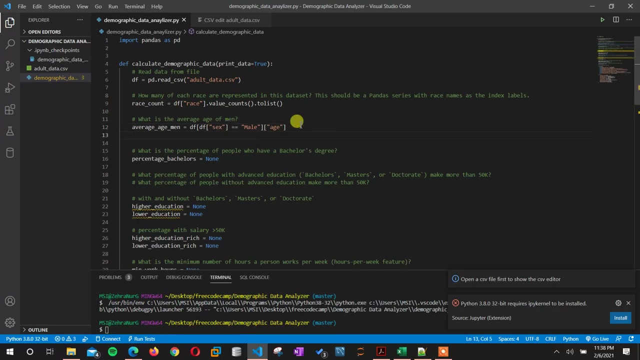 thing is: just look at the, it's big, big character or small, okay. so let's say: okay, this is equal male, right, okay? so then i will take my h and i mean i just go another line and i can use here numpy. okay for the mean import numpy. 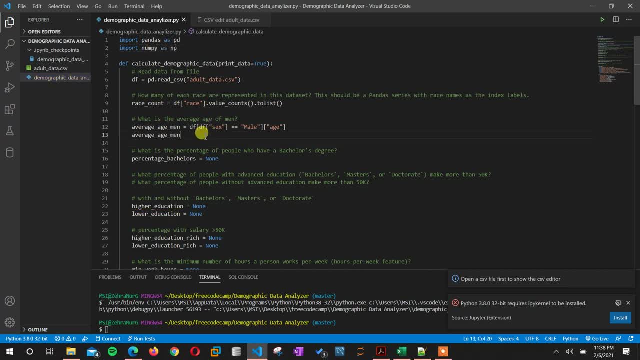 um, so there you go, numpy mean, and i want this. that was here, so it will actually find the mean of this one. actually they found these value in a rounded okay, so I'm just going here write round and I will say, okay, just one decimal, so that's it. just check it, you found. 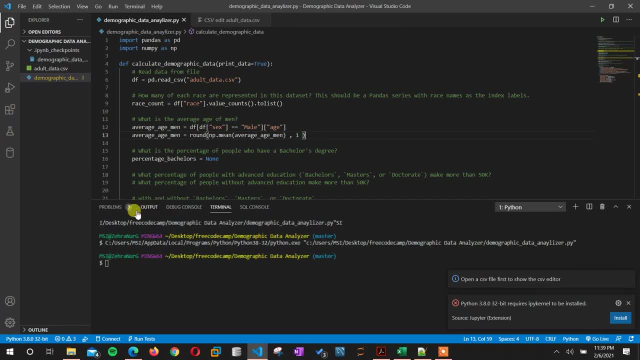 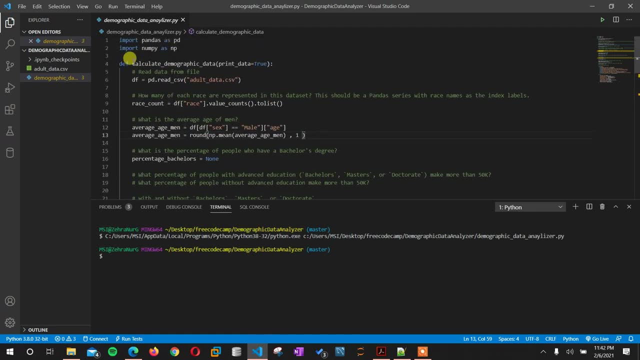 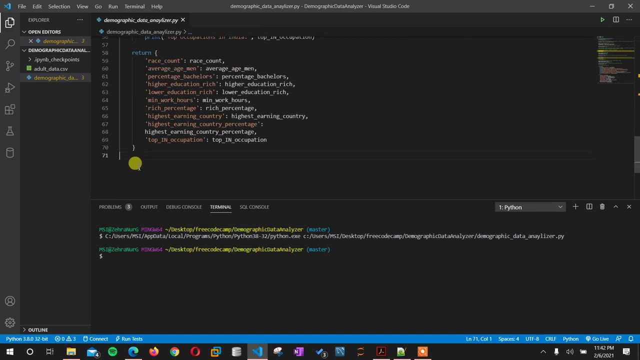 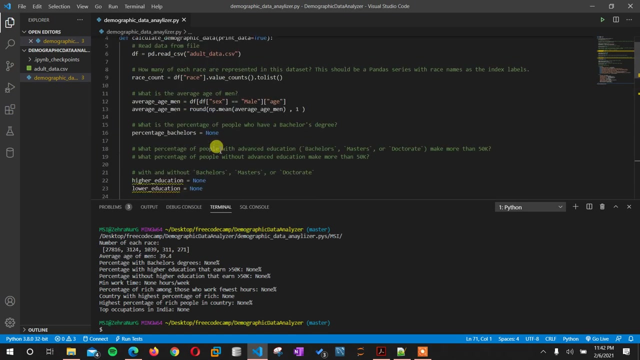 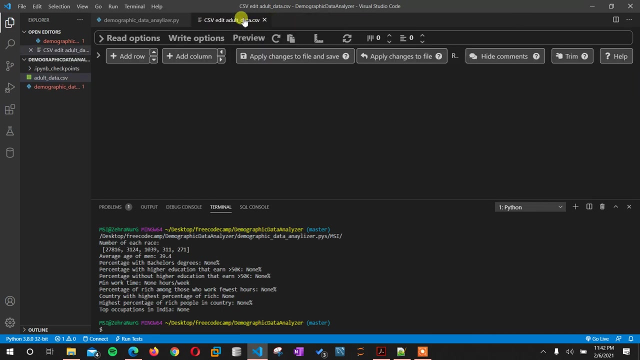 something or not? okay, okay, it didn't happen because I actually forget to call the my. okay, well, in here it will work now, yeah, we find the average of domain as you want. okay, so what is the percentage of people who have a bachelor's centigrade? so that's a find the personally my column here. so okay, here's. 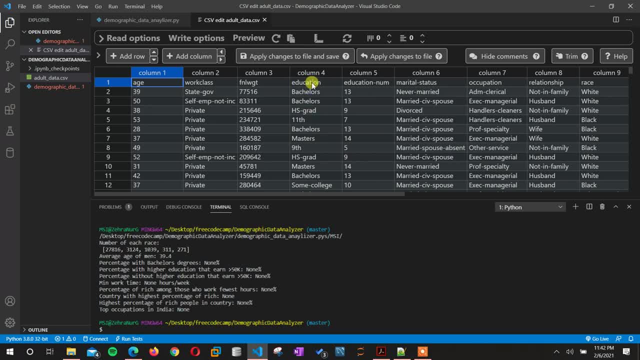 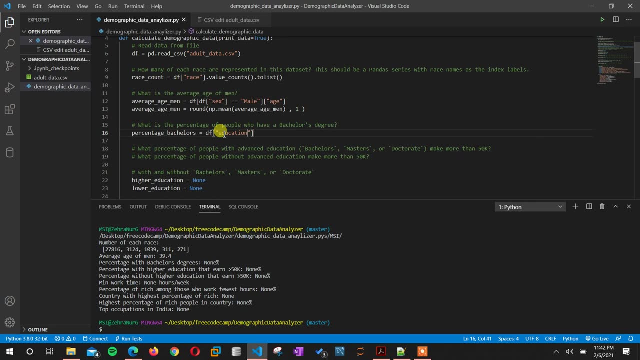 the education: bachelors, bachelor's. it's going like that. okay, so I'm gonna use the name of this column. so, DF, you find my column where I'm that us here and I will take the length of this one using it and actually I will say here: okay for the bachelors degree. I. 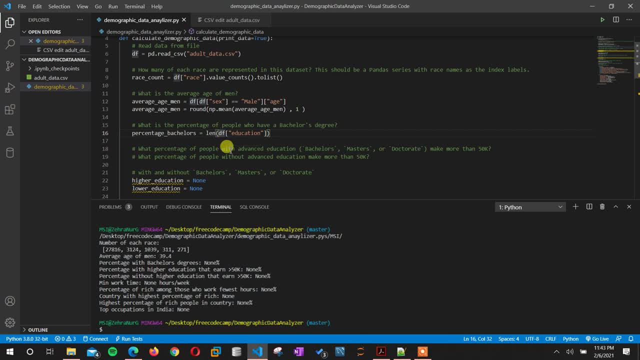 can actually do something like that idea again and I want to just find bachelors, okay, in parentheses, so it actually finishes okay. so what about my total education? I just need this, yes, and then take the length of this one. so maybe you can find another solution for this question, but for me it's the simple way. so for the 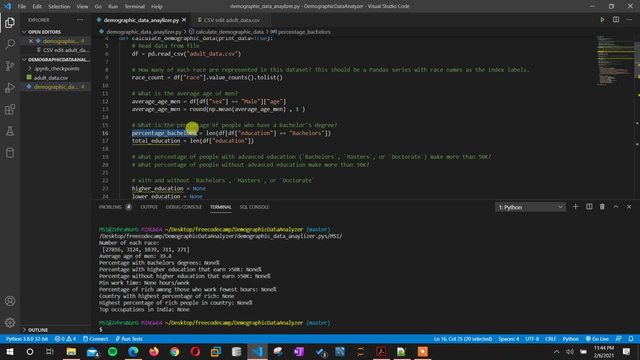 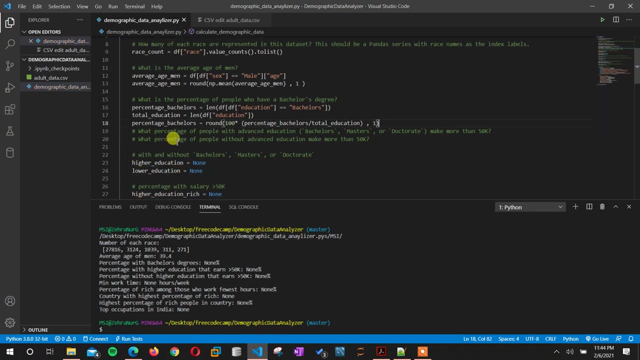 percentage bachelors. I want to say okay, percentage bachelors divided by total education. so I will again round it, because when we are going to test this cause, I don't want to see an error, okay. so yes, just one decimal, it should. so another question: what percentage of people with advanced? 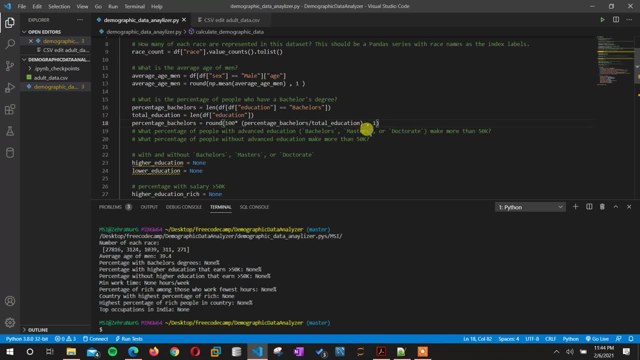 education. give bachelors my stars or another, make more than 50,000. okay, so actually I taught a little bit. I'm gonna write the code here. okay, I actually took. maybe I can do it like that. hey, I can use the lock for finding the index, okay, so, idea of education and to drink, which is which? 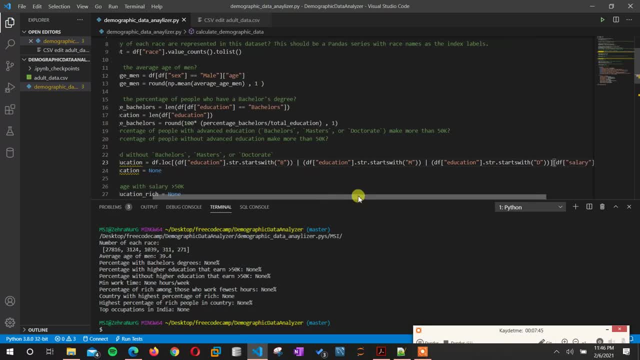 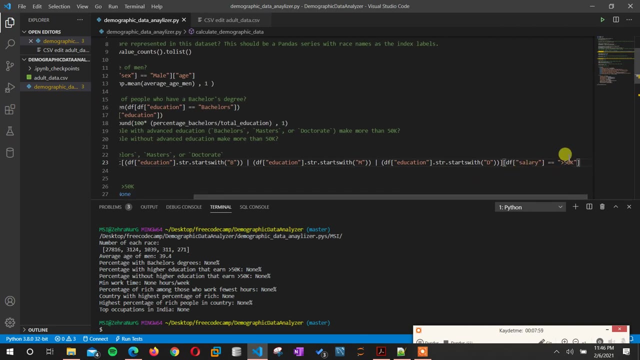 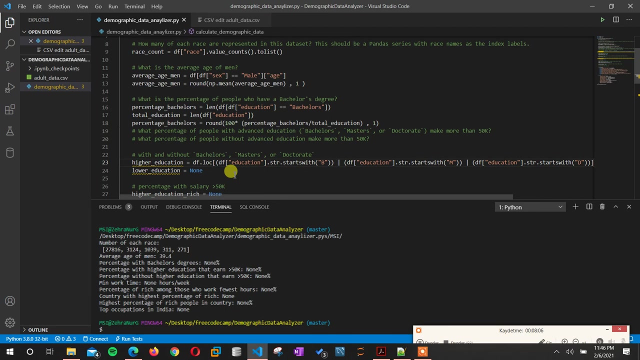 starts with B, I mean bachelors, and M and D, not, and actually this is or or, okay. so then after that I say: but they should get a salary with this one number, okay, so that's it. I will pass the lower education for now. I will say: who have? 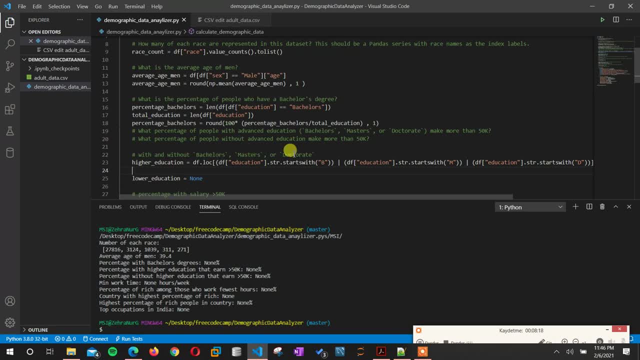 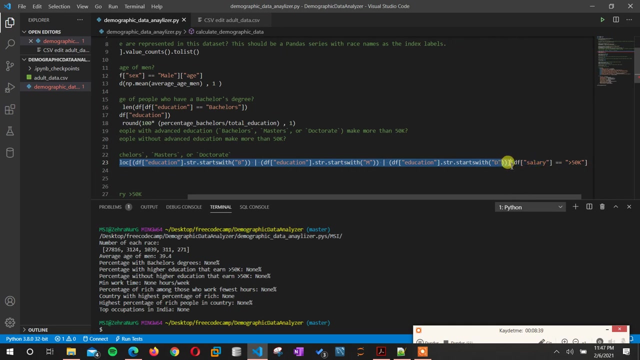 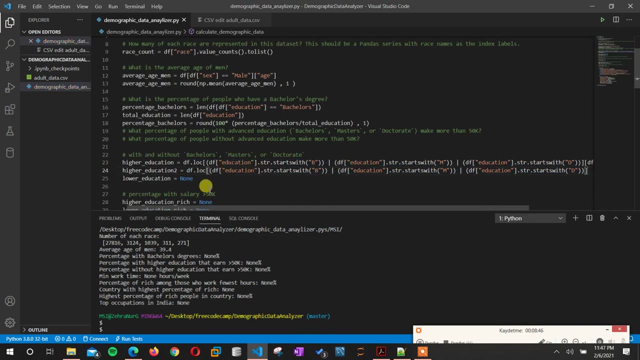 actually degree of bachelors, masters, but they actually can get bigger than 50 or smaller, smaller than 50. okay, so higher education, this will be the second one, but i will just take it from here to here. okay, so take it. yes, so we can find it. now, our percentage like the? 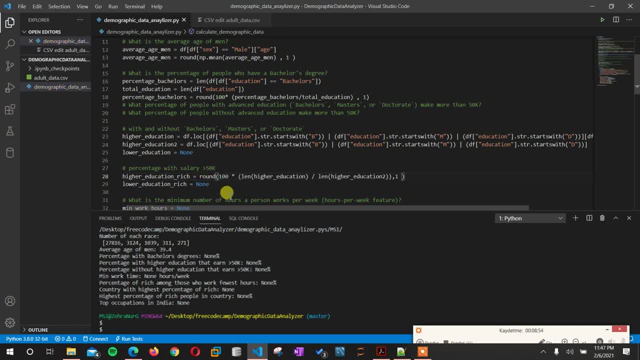 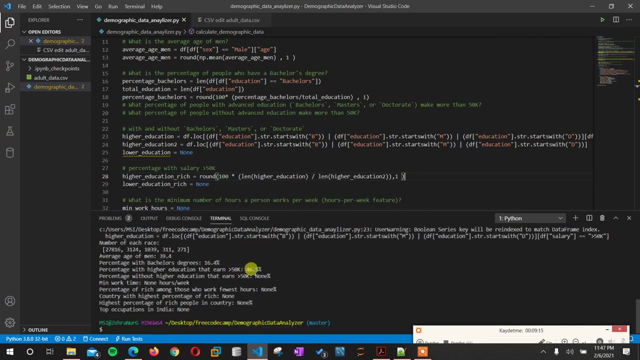 before one. okay, i run it and also i again rounded this number, so length of the higher education and length of the second higher education, and then i take the just one decimal, okay, so actually we can see the answer from here. we should find, uh, just this percentage. 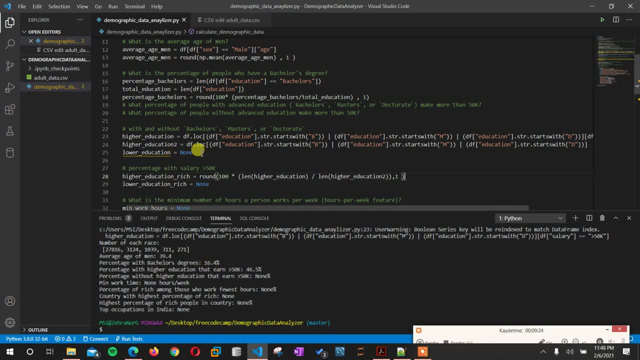 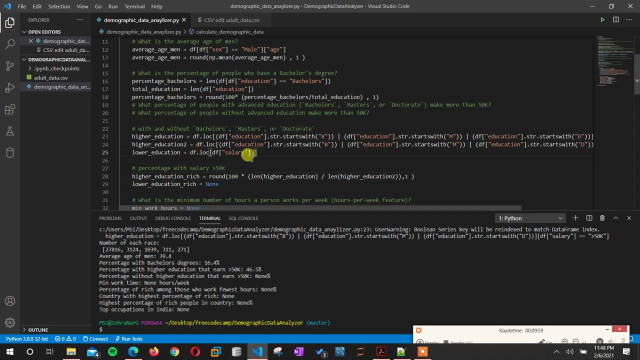 of 16. okay so, lower education: actually similar, but I actually want to show a different way. so I firstly wanna look at the, your idea, look and idea, then shall we get the salary. okay, so, and I will find the look and idea, then shall we get the. 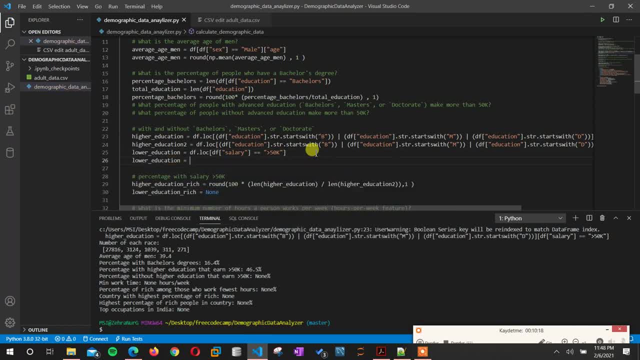 lower education as like that. okay, give me the first number of this one, okay. so actually this is the. this actually has the all of the education degrees, right? so lower education, okay, and I don't actually suffer from the range of the higher education who actually have bachelor's, master's or doctorate, so you, 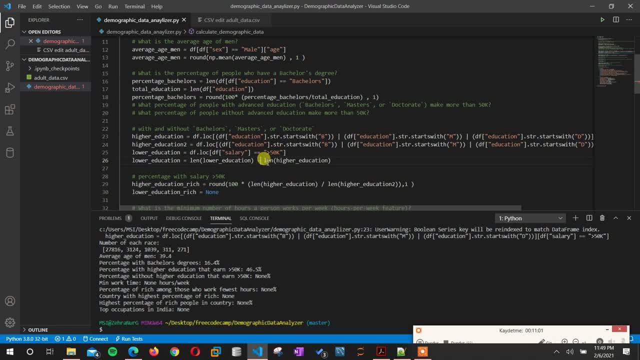 can now find: okay, this is minus. you can now find the lower education degree, and you can now find the lower education degree and you can now find the lower education. right, this is total. this is just what I don't want. okay, so now, this is the very 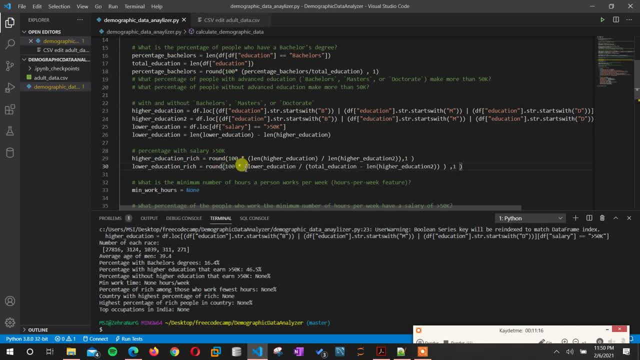 easy question now. okay, here, I actually find the lower education okay, as they want, but actually I've found the whole education also here, total education, right. so I wrote it and then I said, okay, minus higher education too. okay, so you can now find the percentage of these. 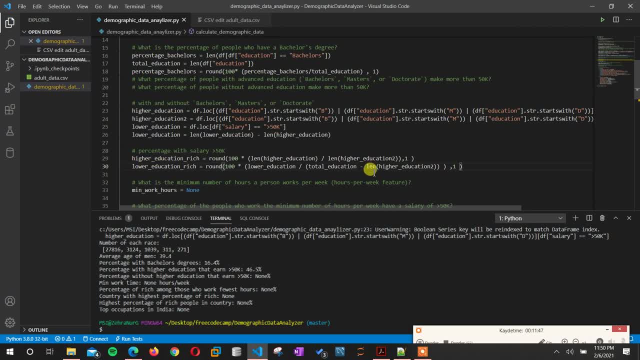 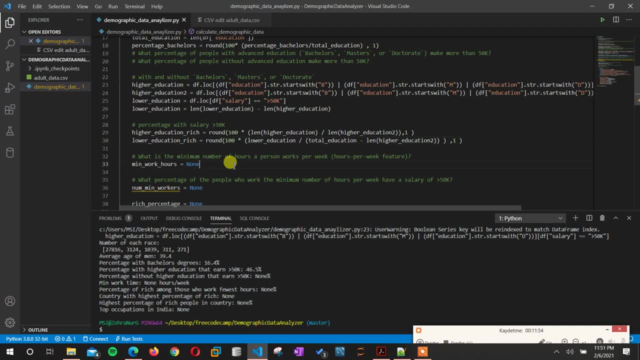 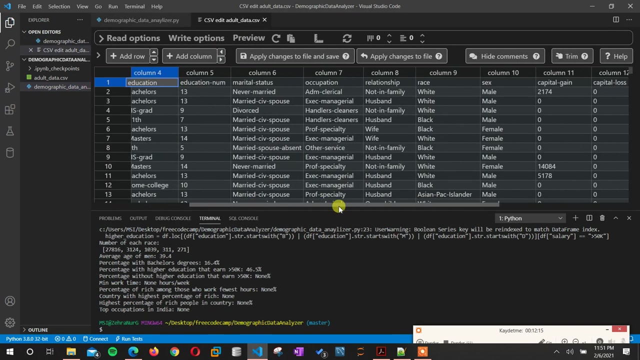 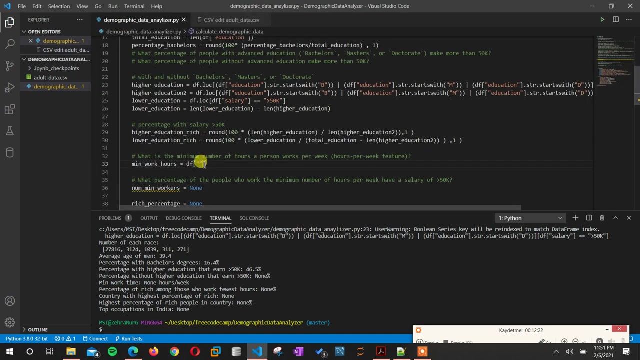 lower education, rich people. okay, next questions: what is the minimum number of hours a person works per week? so let's think of it. we actually can use minimum here. so I'm gonna write the idea: find okay, what is it name here? yes, hours per week, and that's it. then I will say just okay, so we can see it now. what's the number? 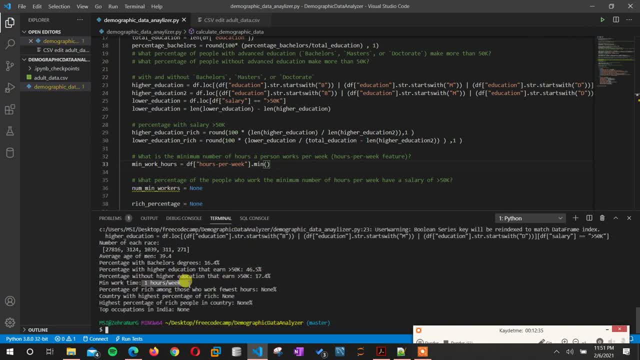 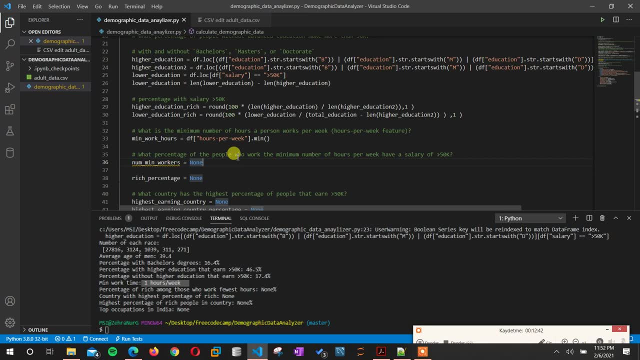 of it. so here, one hours per week, okay. so then they ask what percentage of the people who work the minimum number of hours per week have a salary, and then they will get it actually than 50,000, okay. so now, actually, I know the minimum hours is the one, all right. 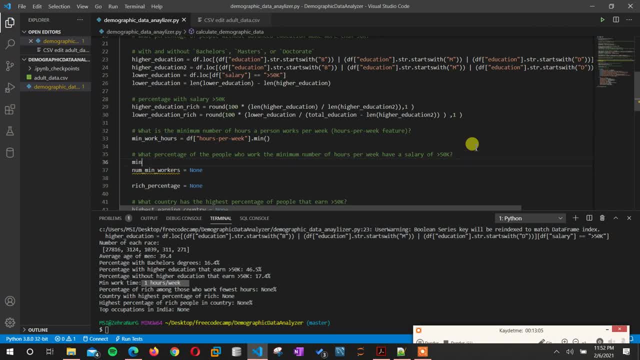 so I will say so: minimum work and DF- I'm searching hours per week, okay so, and I want it, it should be equal to do one, okay so then number of workers: hey, yeah, that's look then what I will say here. okay, we can actually take it from here, yes, and I want to say, hey, I should use you and 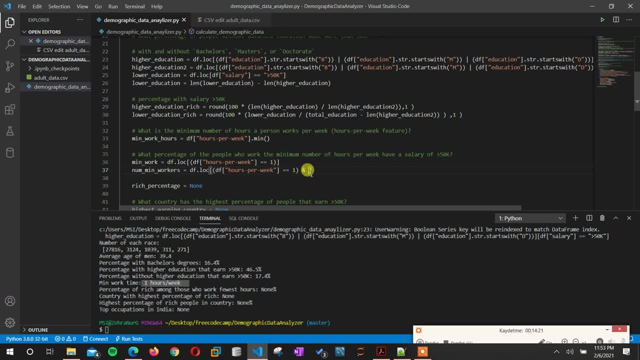 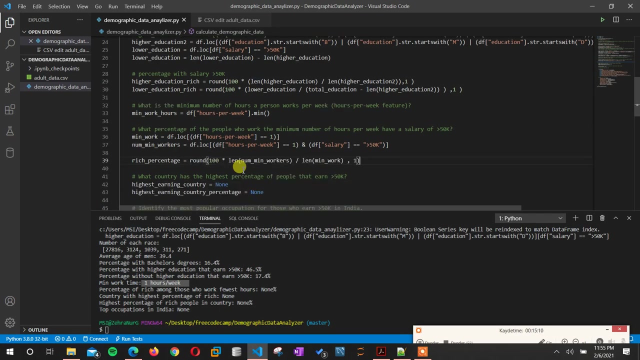 operator, then I should say it should be actually solid condition. take the seller cognition clear. so now I can find the fridge percentage. so hey, plan number of minimum workers and over range you work okay. so actually again I'm going to run with this number and that's it so. normally, of course, I taught 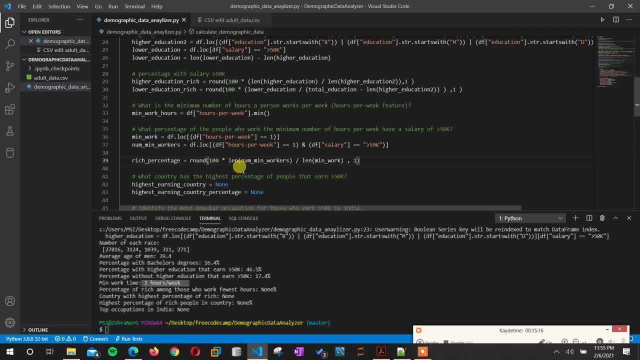 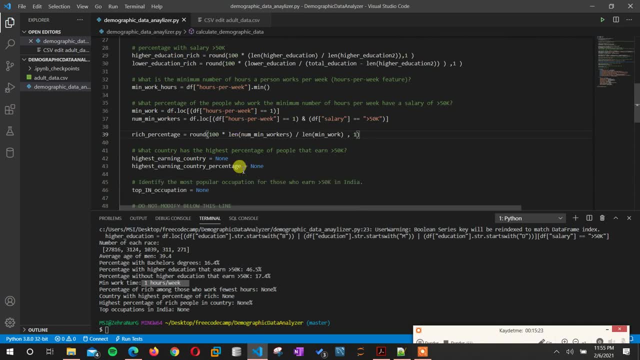 these questions before, okay, so just don't look at the answers and try some way and then get help from here. so the other question: what country has the highest percentage of people that earn bigger than 50? okay, so they want actually a country name, also the percentage. okay, I think this is. 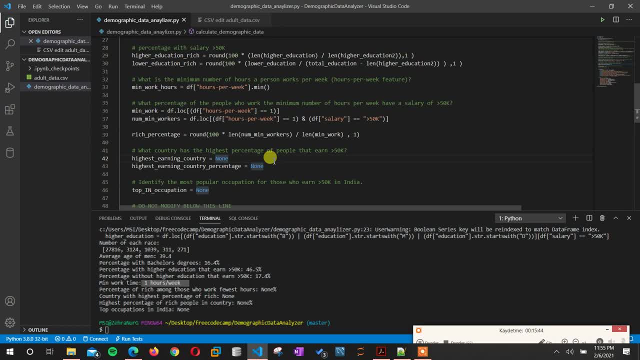 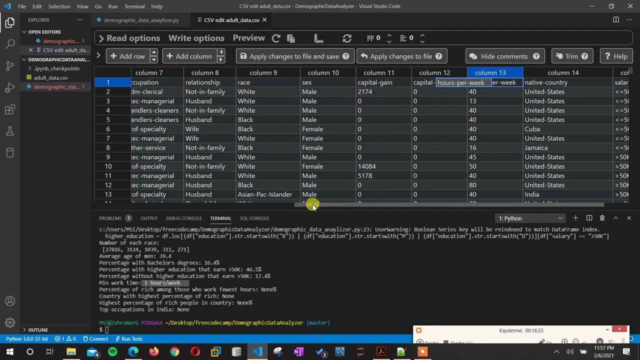 the hardest problem in here, okay. so what I'm gonna do here, I actually find right here. I need the app and look again, I actually take this condition, okay. so then I want to find the country. but let's check it, the countries, where is it? yes, okay, native country, okay. 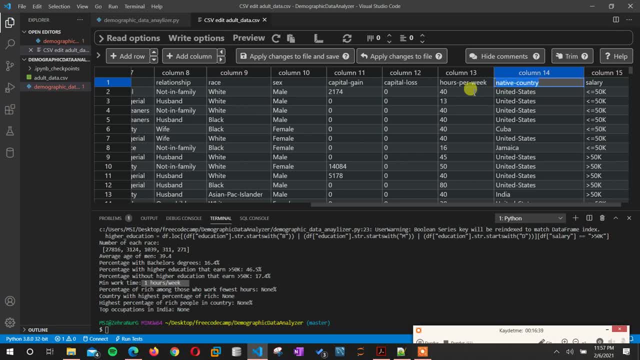 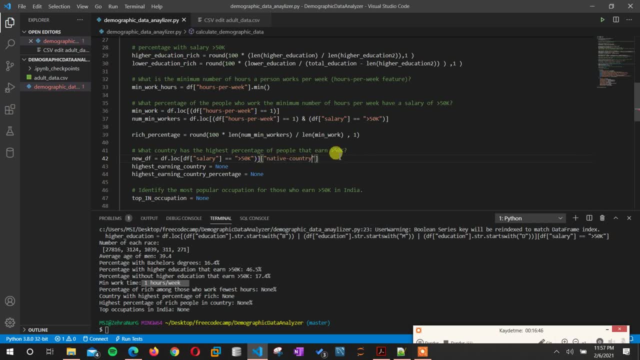 these are country. so, yes, native country find and then actually get this one fit together. okay. so after that I just want to find this one native country, but they don't have to take and salary bigger than 50. okay, so again I will say value because it can put together the same country. so now, actually the hardest part finished, okay, so I. 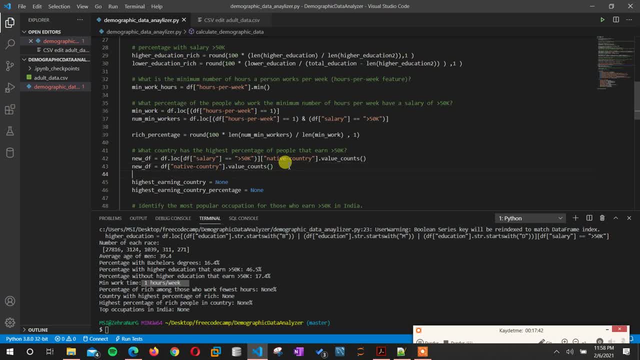 will actually want to find what is the maximum percentage in here. okay, now I can find the country like that, but after that I should find the percentage okay. so maybe we can find firstly country. okay, here I will divide new df over new df2 so I want to say, hey, sort my values and I will use the 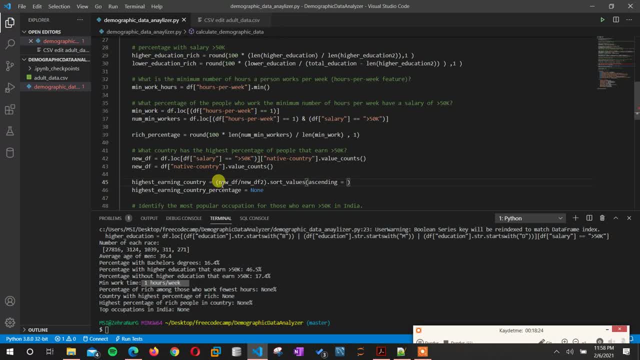 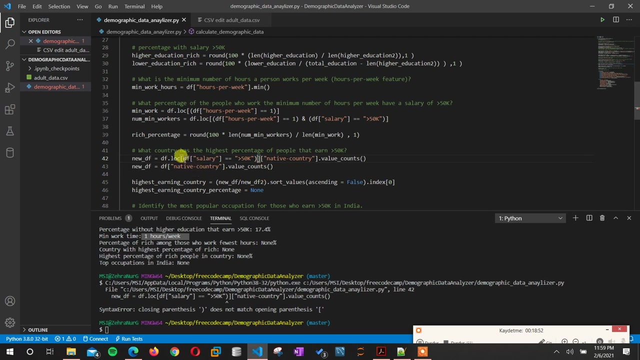 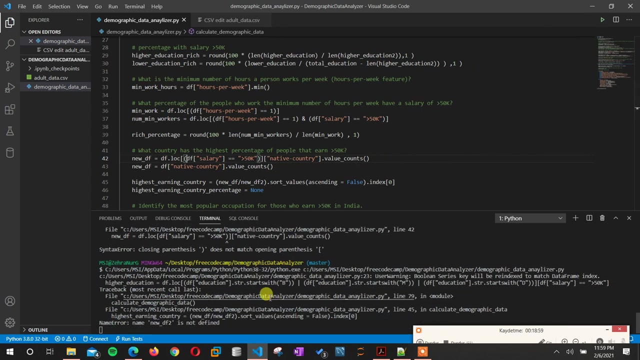 ascending it should be, so I can see the highest earning country. okay, so, and I will take the first one, so I say index 0. okay, it finished, we can see which one. there's a mistake? okay, we can use your another contest. okay, so start. I forget the number. 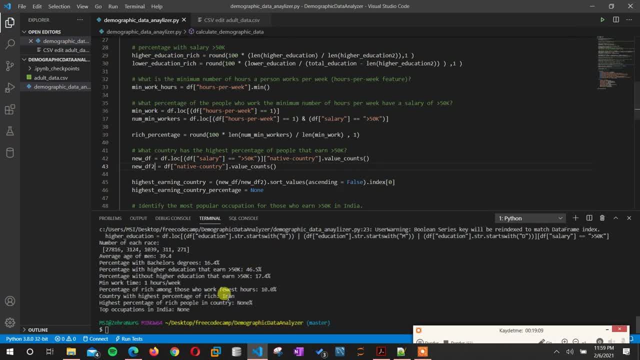 okay, start. yes, the highest, actually percentage of the rich country is iron, okay, interesting. okay, now we should find the percentage, exactly a number we should find. so let's say, hey, richest should equal me, and now find my which is and maximum value from here. so you can now right. 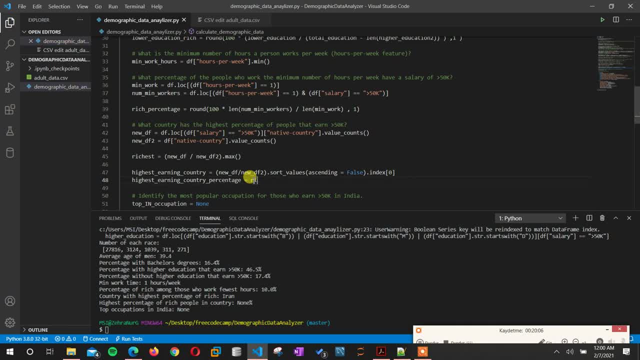 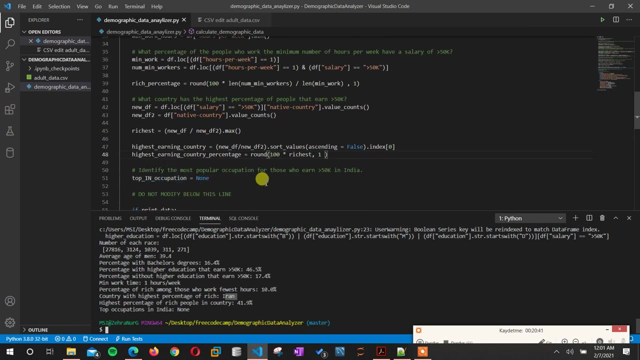 here reaches right, so let's check it got. okay. this is actually belong to do this country right, okay? so last question is here: identify the most popular occupation for those who earn bigger than 50, and we should find people from India, right, okay? so what can I do? 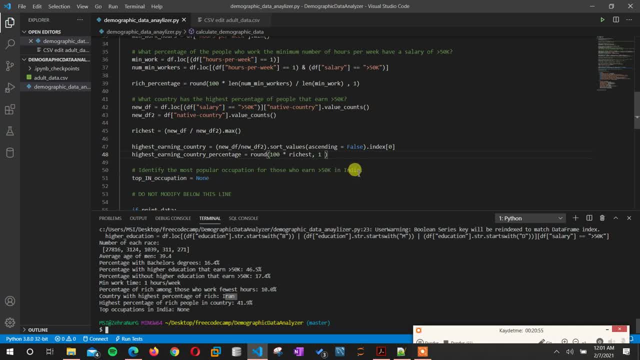 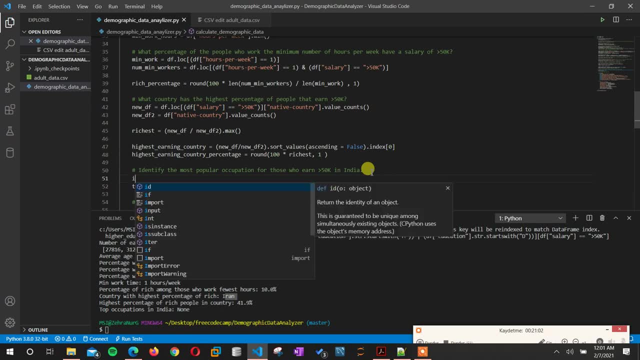 here I actually just find in-veh country and occupation column. okay, let's try it in India. yeah, that's good, I'm gonna make sure I have my new path perfect. so, okay, look, and then the app. I'm not going to do it again, it will be the same, and also: 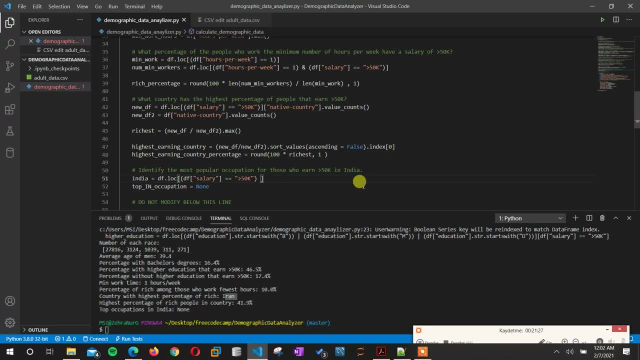 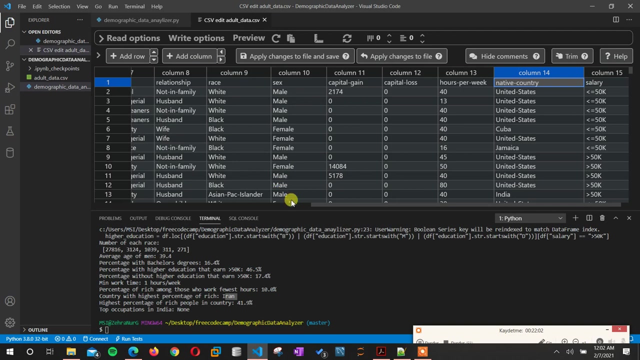 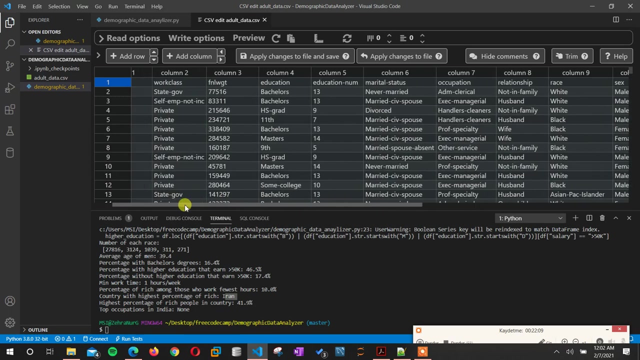 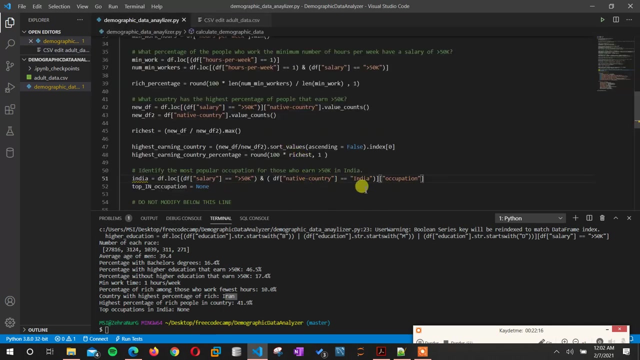 I will use the and operator here and I will say, hey, yeah, choose my column of native country and it should be equal India. okay, then I will say: find their occupation. let's check it, is the true column name or not? where is the occupation? yes, so occupation here. okay, so it will find country and and their. 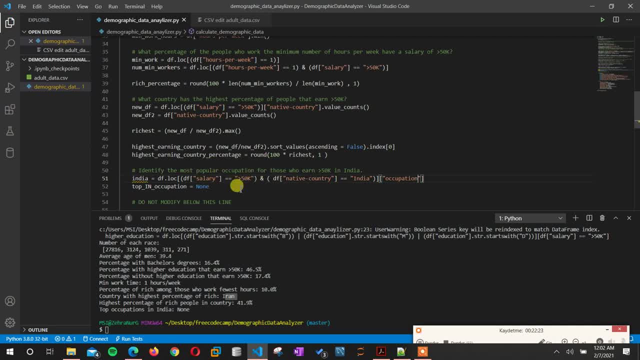 salary with this condition and they, it will find also their job okay. so I will actually want to use here much. so what should I write to first part? maybe not from the statistic, but I can say: did yeah, this size into this cell. so that's it. we actually finish it. yes, this is it. 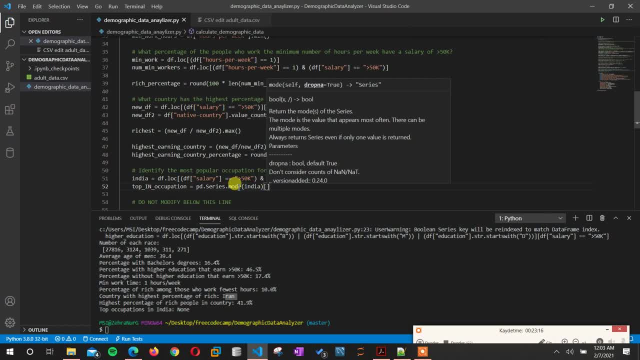 come on, okay, I think it works here. we got it in this section and I want to use it here. I also have to interact with wildlife, which means you guys can listen to this program. I don't want to do any kind of effects or things like that. I want to. 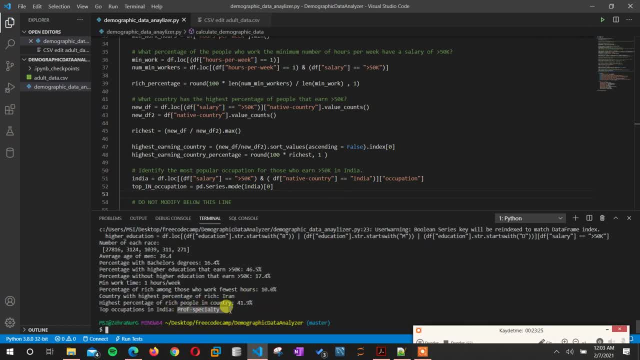 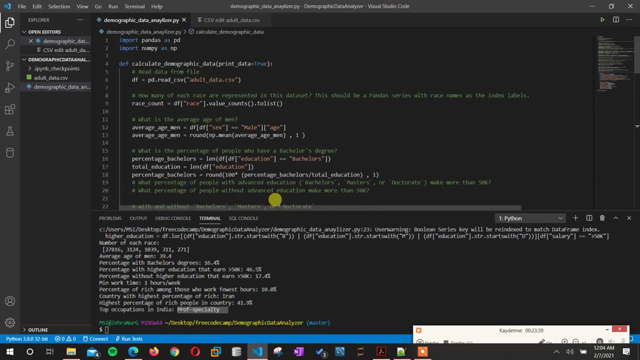 Di rent the house, because my presentation in this video is freaking hard. so you is the prof specialty. this is the top occupations in india and they are actually. they actually get this salary. and we finish all of the questions. so let's check these are true or not. from the